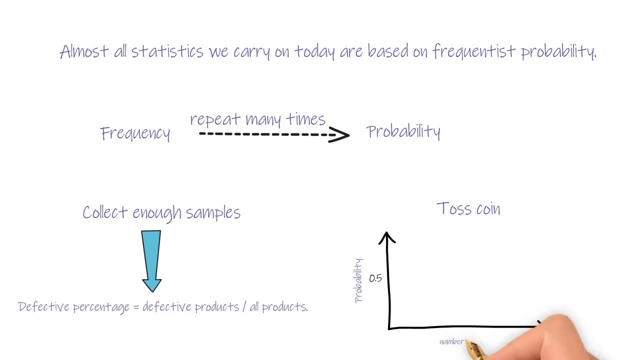 probability of every event. As long as we do enough trials, the frequency of that event is approaching the probability of it. The idea of repeating the random event many times and use the frequency of it to reveal its probability is easy to understand. However, maybe you have the doubt that frequency and probability are two totally different concepts. 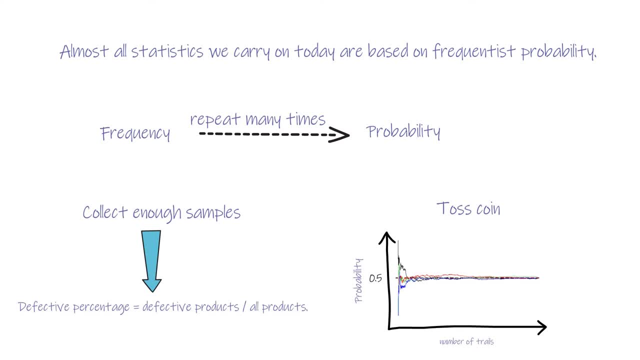 How can you confidently apply this theory to measure all random events? To answer this question, let me do an experiment. TOSA coin, TOSA I get head. Can I see the probability of head is 100%? Of course not. I haven't repeated it for enough times. So, TOSA coin, 10 times 8 head and 2 tails. 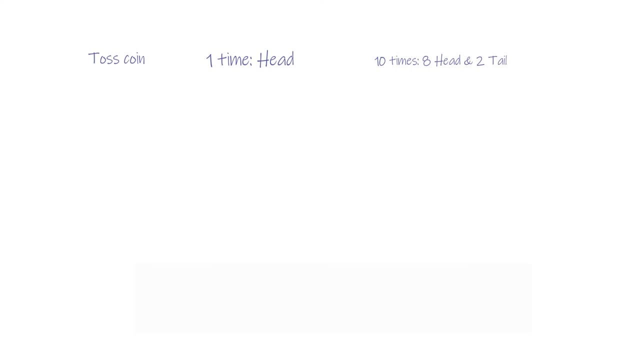 Still not 50-50, as we expected. Shall we continue? Hold on, Actually, many people have already done this before. A big thanks to them for the hard work. Now we can see that it is about 50%. I think most of you may be satisfied with the conclusion and comfortably apply it to: 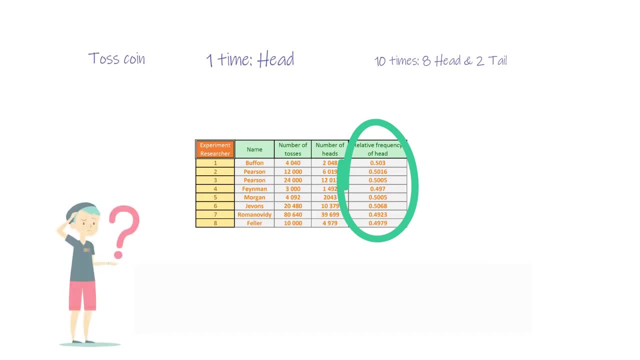 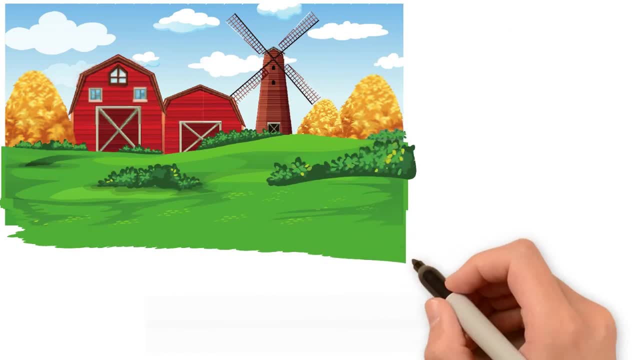 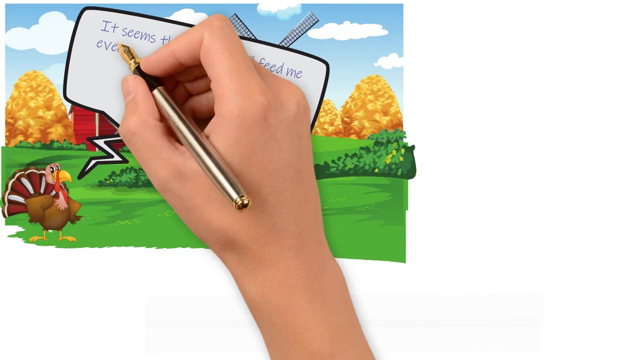 TOSA coin. TOSA coin. Do you know the turkey story? On the farm there is a smart turkey which, good at observation and deduction, It finds out there will be a farmer who bring food every morning. The turkey thinks it seems that farmer will feed me every morning. But I won't rush to that conclusion. 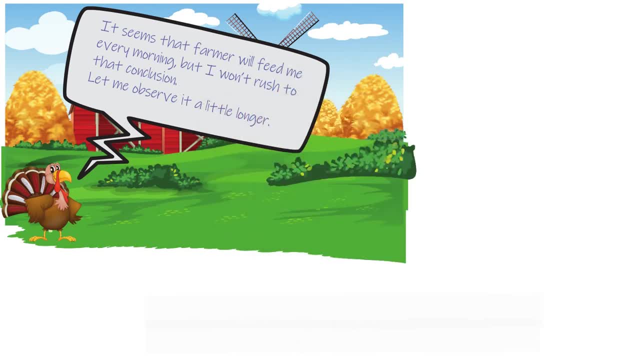 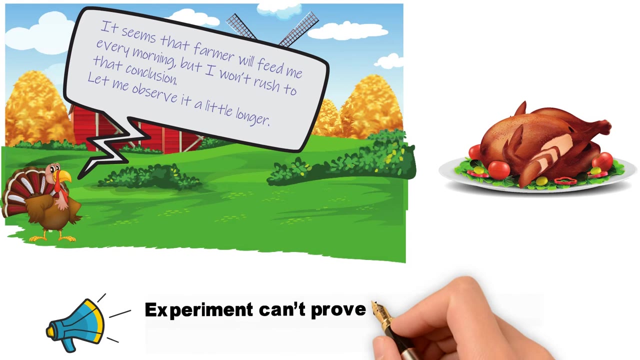 Let me observe it a little longer. So a year later, the smart turkey finally comfortable get the conclusion that There will be food every morning. This conclusion remains true until the Thanksgiving Experiment can't prove the theory is right. It can only be used to prove it was wrong. We need mathematical approval. 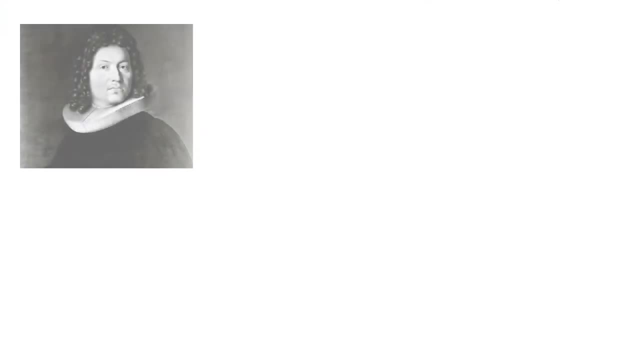 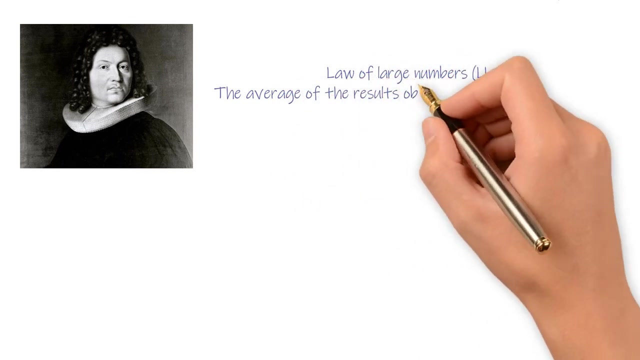 Luckily, this theory has been proved. In 1713, Swiss mathematician Bernoulli, after 20 years of hard work, proved this theorem in his book Law of Large Number. The average, The average of the result obtained from a large number of trials, should be close to expected. 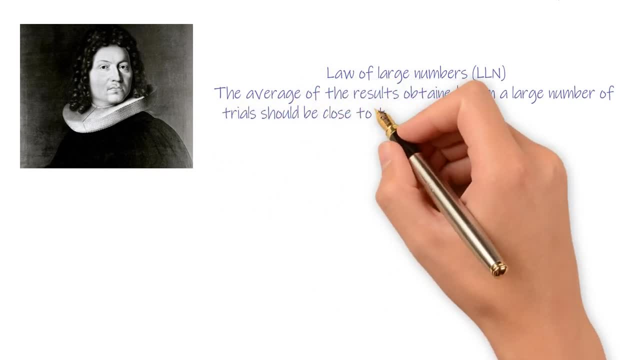 value and will tend to become closer to the expected value as more trials are performed. The Law of Large Number is the keystone of statistic and probability because it guarantees stable, long term results from the averages of random events. Because of it, we can know. 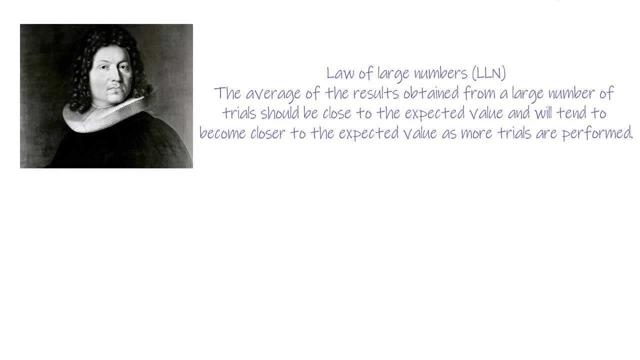 for sure that it is correct to use frequency to estimate, to estimate the probability. Further, under the same condition, using the historical data to predict the future is possible. It opens a door for us to understand the world. You may notice, using frequency to estimate probability. 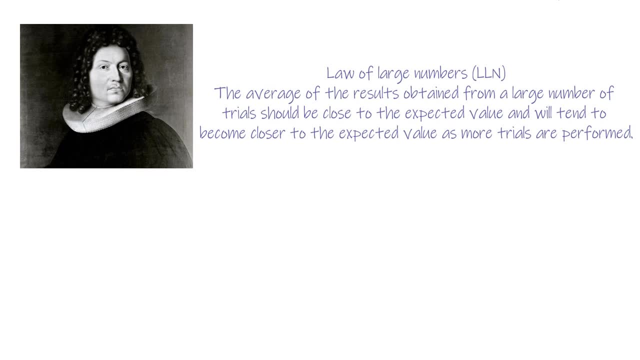 is under one condition, which is repeat the trial many times. So how many times is enough? Ideally, many times equal to approach infinity. But infinity is a mathematical idea. We can't achieve it in the real world. Therefore, in order to use it, 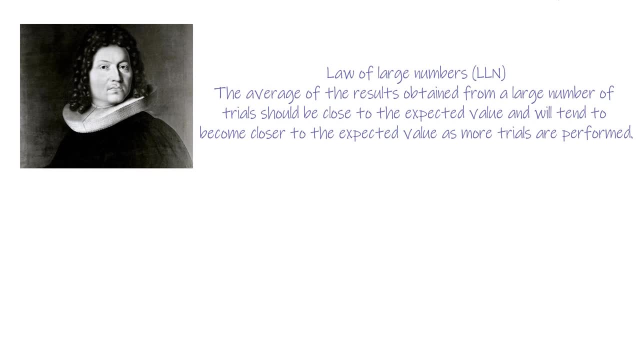 we introduce another two concepts to assist confidence: coefficient and margin of error. The law of large number tells us: more trials performed, the frequency will tend to become closer to the probability. In another word, the value of frequency will bound. It has a range around the value of the probability. 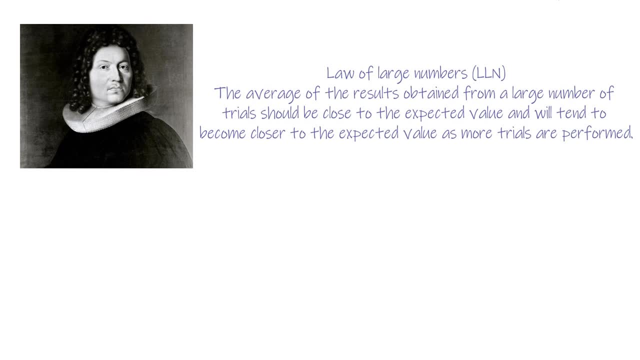 This range is the margin of error. For example, Tosa coin: theoretically there will be 50% head. If from an experiment the relative frequency of head is 52% to 48%, then we can see the margin of error is 2%.